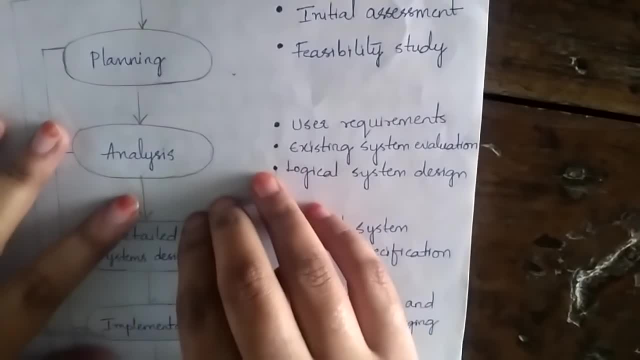 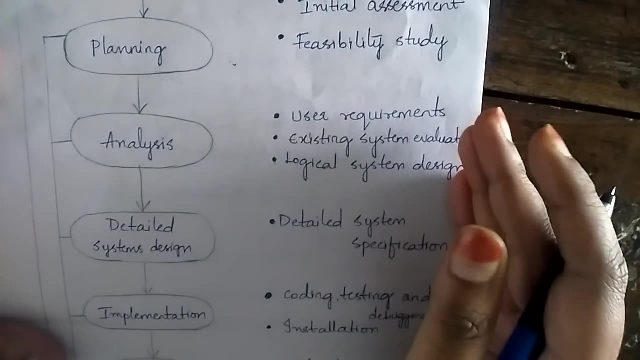 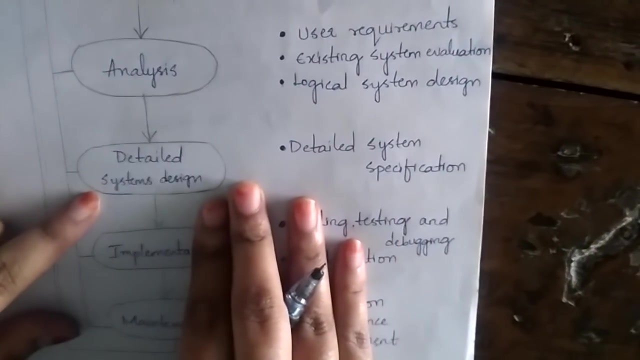 study during the analysis phase. The result of analysis should be a better understanding of the systems, functional areas, actual and potential problems and opportunities. The analysis phase also includes the creation of a logical system design. Next comes to detailed system design, detailed system specifications. In this phase the designer completes the 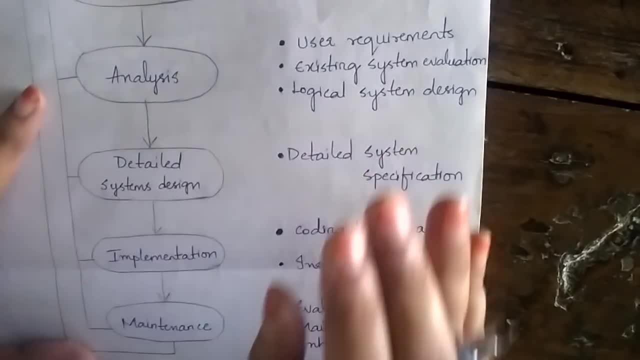 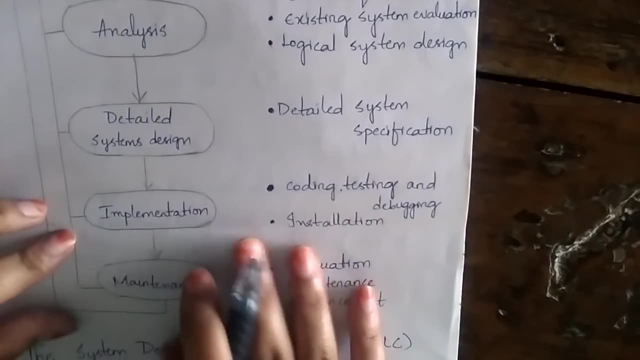 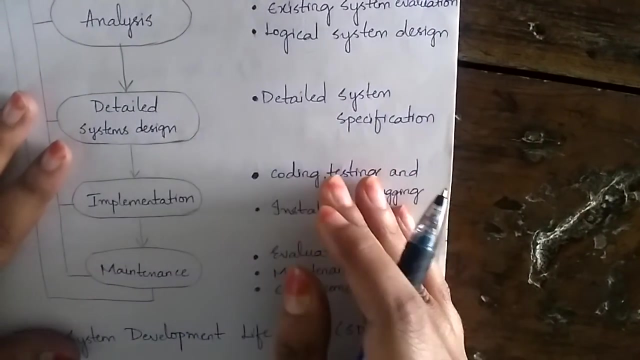 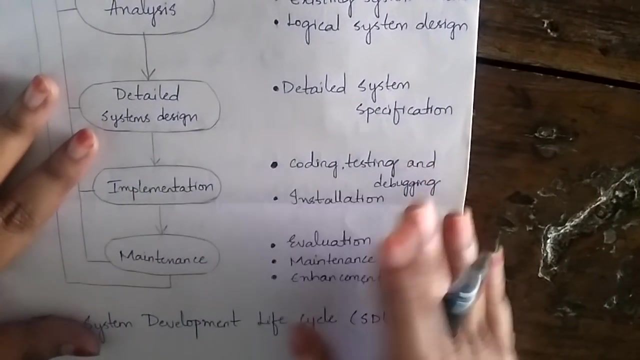 design of the systems process. It includes all necessary technical specifications for screen menus, reports and other devices. Next comes to implementation, implying all these things: During the implementation phase, the hardware, DBMS, software and application programs are installed and the database design is implemented During the initial stages. 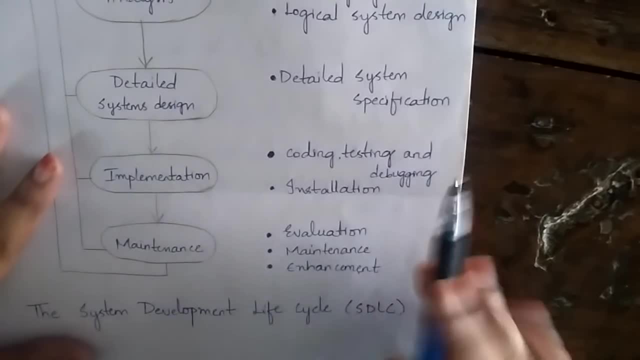 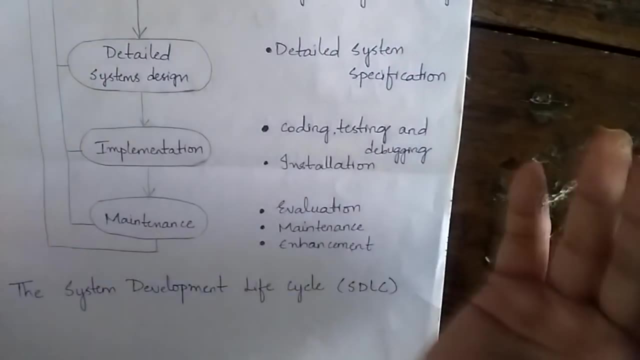 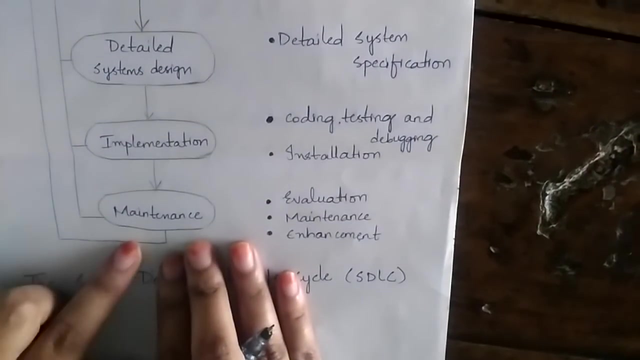 of the implementation phase, the system enters into a cycle of coding, testing and debugging until it is ready to be delivered. After testing is concluded, the final documentation is reviewed and printed out. The system will be continuously evaluated and fine-tuned for better performance. Next, Maintenance: Maintenance almost as soon as the system is operational. 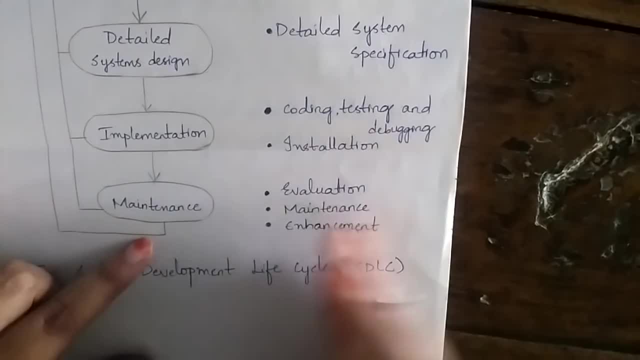 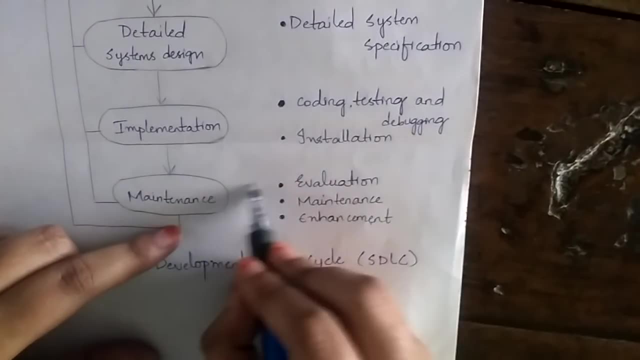 end users begins to request changes in it. Maintenance is of three types, ie Corrective Maintenance, Corrective Maintenance, Adaptive Maintenance and Perfective Maintenance. In the Corrective Maintenance, corrective maintenance is used in response to system errors, IF the 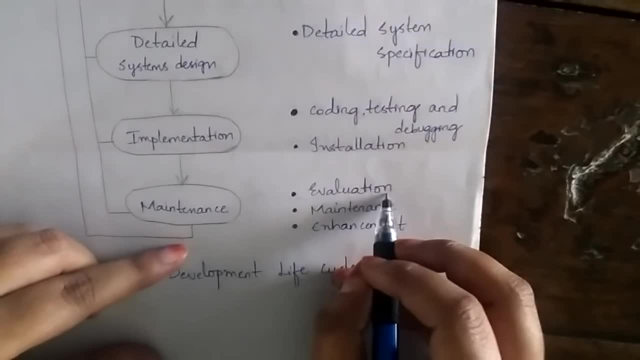 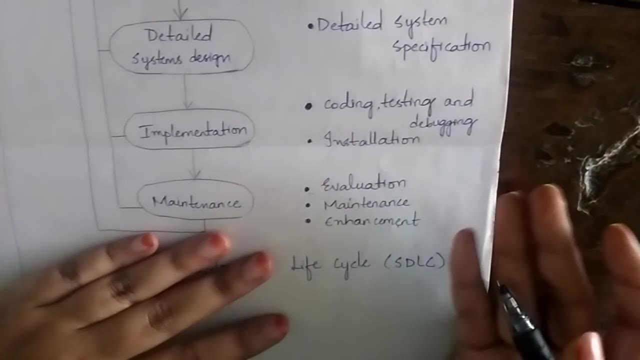 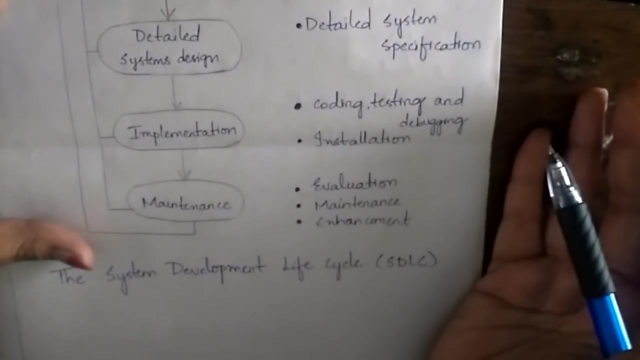 system get any error, then for some social sources or being left at home for certain, maintaining the errors, we use the corrective maintenance, then adaptive maintenance. It changes due to the changes in the business environment. Perfective maintenance is to enhance the system. So this is all about system development life cycle. Thank you.